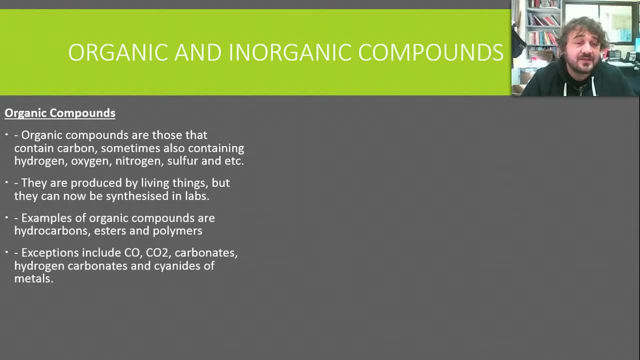 carbon dioxide carbonates, hydrogen carbonates, cyanides of metals. these are not organic compounds. So they look like organic compounds, but you need to understand that list of exceptions. So what are inorganic compounds? Well, they're just anything essentially that's not organic. 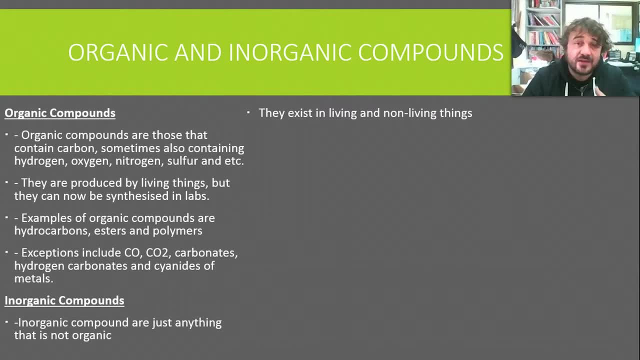 So they exist in both living and non-living things. Water is an inorganic compound. Sodium chloride is an inorganic compound. The main examples that we talk about are water, acids, bases and salts. So how do we test them? How do we work out what's what? Well, so we get. 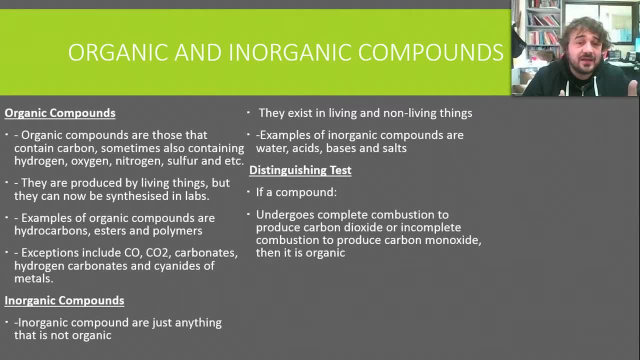 a compound and we burn it. Now, when we're burning it, if it's complete combustion and it produces carbon dioxide, then we're going to burn it. So we're going to burn it. and if it produces carbon dioxide or carbon monoxide, then it's organic. So only organic compounds. 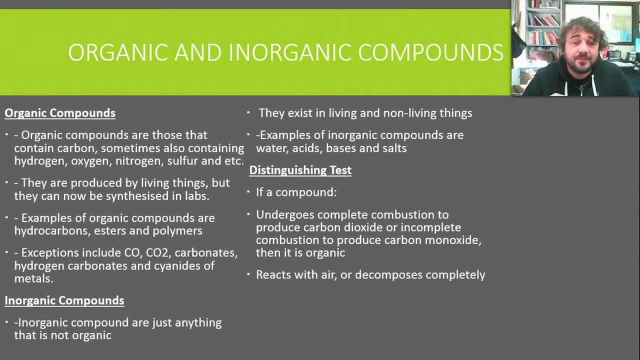 produce carbon monoxide or carbon dioxide when we burn it. They also react with air and can decompose completely. So if it does these, then it's most certainly organic. So when a metal reacts with air, it oxidizes, but it won't decompose completely. It'll make. 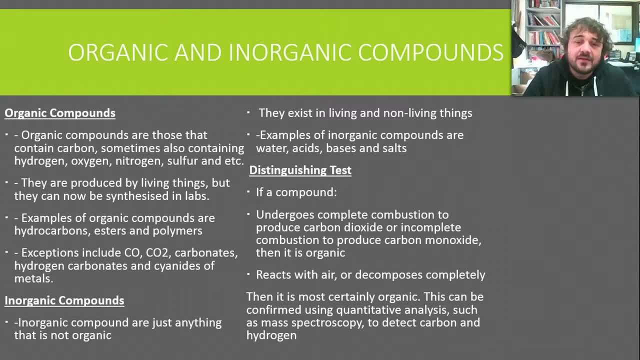 something new. It'll vaporize off into the atmosphere. So we can then confirm these using quantitative tests like so, mass spectroscopy, And if we do this, so if we do some mass spectroscopy- we can determine if it has carbon and hydrogen in it. All right, we'll talk more about that. 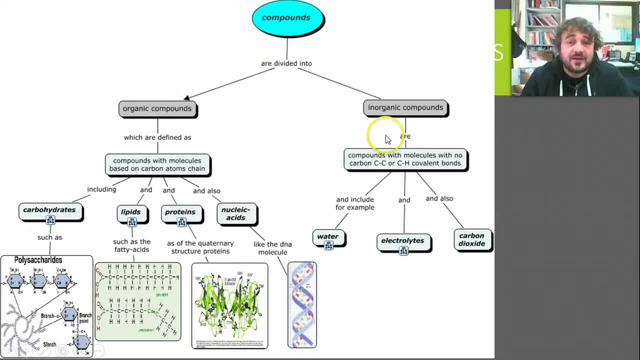 sort of stuff in a minute. So basically we divide our compounds into two types and here's a little flow chart for you. So it's inorganic compounds, Compounds with carbon dioxide molecules with no carbon C-C or carbon C-H covalent bonds. And here are our different. 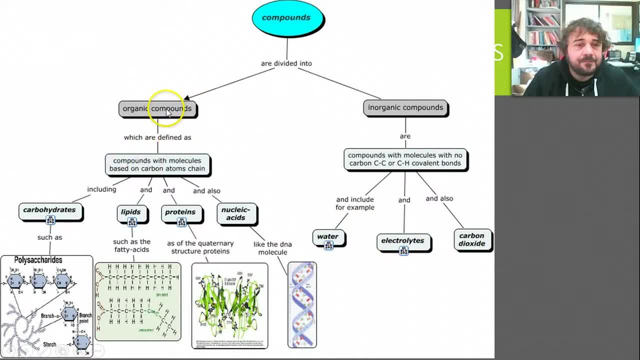 examples, electrolytes being salts. So we've got our inorganic- sorry, our organic- compounds, molecules based on carbon atom chains, and here are several different types, And we'll look at some of the carbohydrates. We've got lipids, We've got proteins that have a lot. 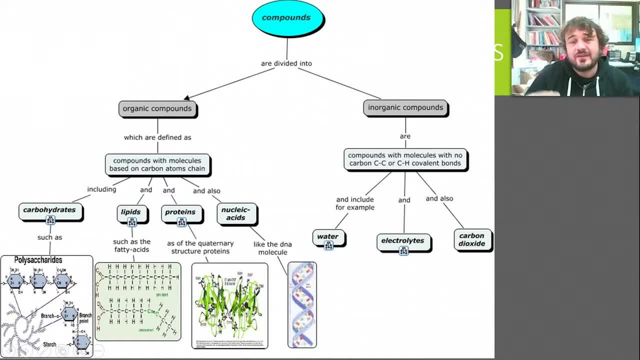 of extra stuff bound into it and have a quaternary structure. So we've got a lot of extra stuff bound into it and have a quaternary structure, And this quaternary structure means that it's got this giant 3D structure that folds around itself And the structure is actually important. 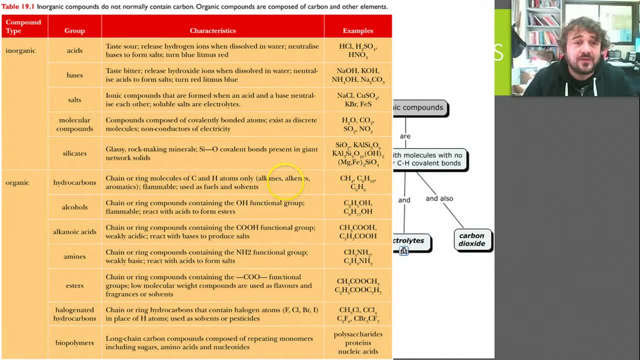 And here's a table. This is a table just from your book, And we've got some characteristics here which can be used to identify them. Okay, we're going to go to those. If you want to write those down, feel free. All right, so let's have a look at our organic compounds. 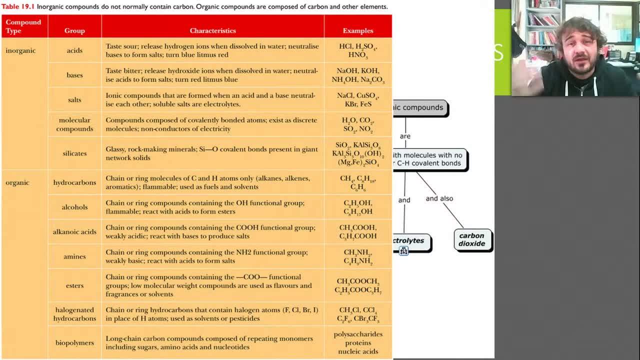 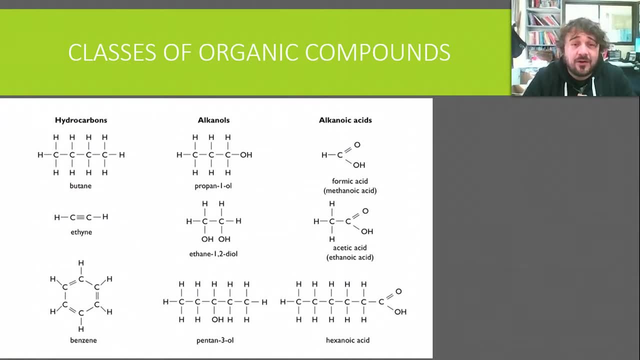 I would know those. by the way, I'm just going to spend time in the video Going through them all for you. So get those sorted, have them in your book. All right. classes of organic compounds. So we've got three that we need to talk about. 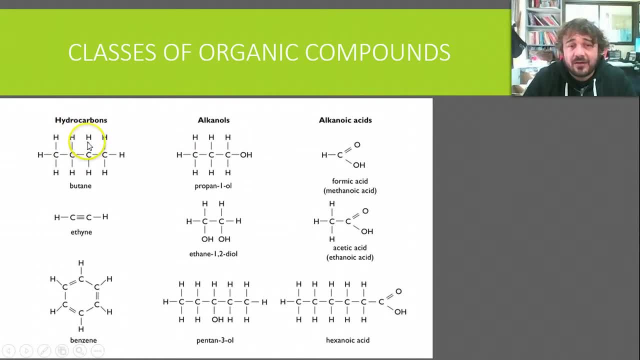 We have hydrocarbons. Okay, these are our alkanes. We have alkanoles, So they have the OH group here. So alkanes, alkenes and alkynes, We have our alkanoles and we have our alkanolic acids. So 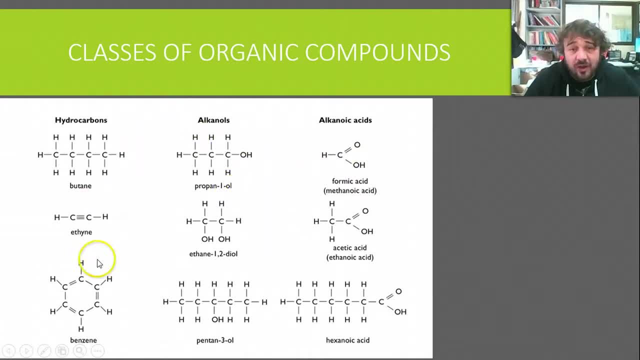 this is again just a bit of revision. You should know how to name these now. This should not be new. Here we have our hydrocarbons, So we've got the ane, the iron, the benzene here- Remember benzene being the toluene ring- We have our alkanoles, which 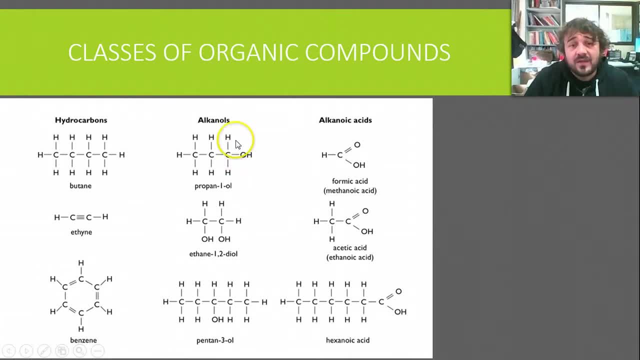 are also alcohols, But we have our alkanoles with the OH group on the side, And over here we have the alkenolic acids. These are my favorites. I like these and I like putting this with that and making an ester. That's my favorite experiment. That's one of my favorite. 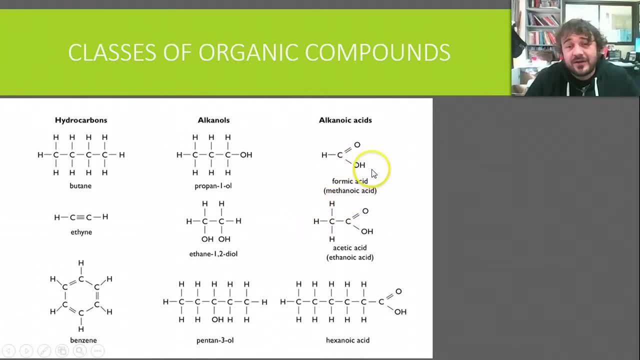 experiments to do in the entire course. So we've got our alkanolic acids and they've got this group here and that group is pretty cool. So you know how they work. That's all revision, essentially. How do we tell which? 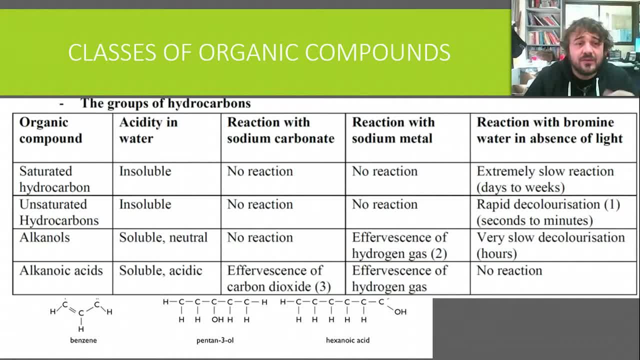 one we have, though. So we've got a saturated hydrocarbon. You need to know this table In water. it's insoluble, so it's neither an acid nor a base. Reacts with sodium carbonate? it doesn't. It does not react with sodium metal, The saturated part there. that means it's holding as many. 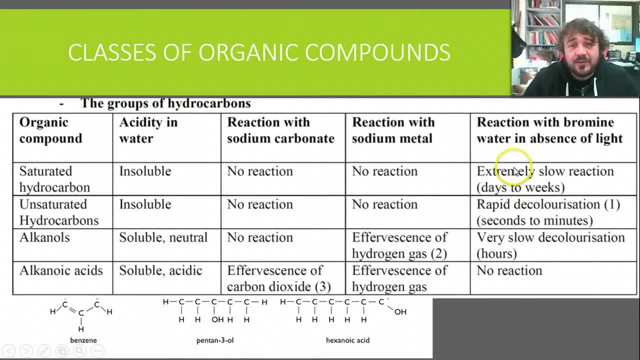 hydrogens as possible, And when we put it with bromine without light, if it does react, it reacts very, very slowly, Whereas our unsaturated hydrocarbons, so our alkenes and alkynes, they are also insoluble, They do not react. They do not react with sodium metal, But with 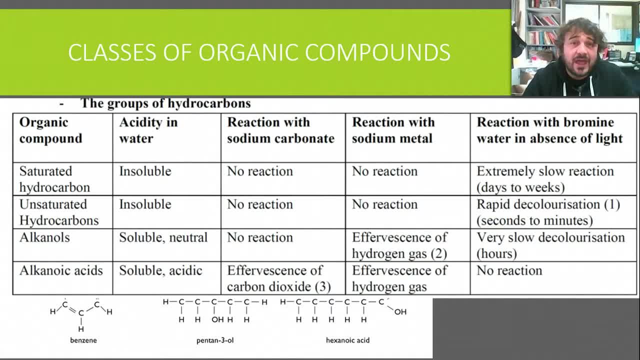 bromine. in the absence of sodium, it does not react with sodium metal. So we've got some contrasting things here. We've got some green lookout dots And you can see that in the absence of light they will react and 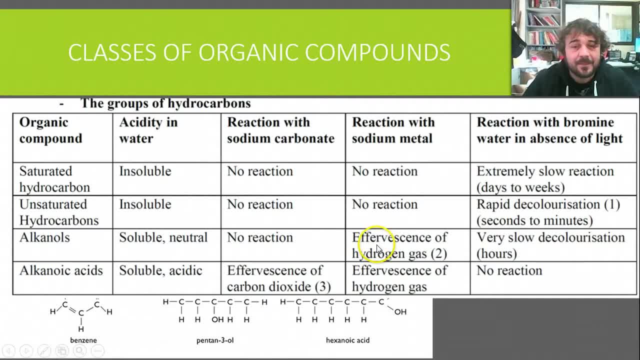 they'll react very, very fast, So they'll lose the color or the bromine will lose its important. we'll see this in a table, in a flow chart, in a minute. they effervesce hydrogen gas if you put them with sodium metal. okay, that's important- and they very slowly, so over hours. 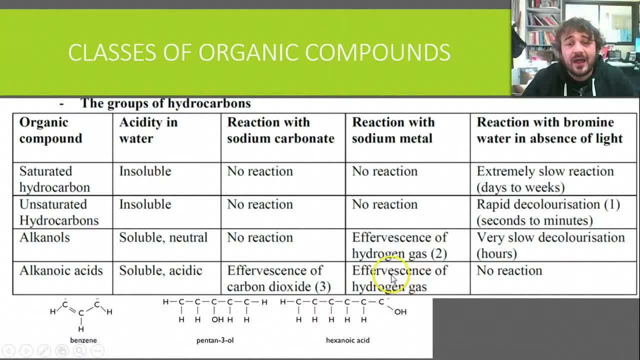 they'll react to the bromine. alkaline gases don't react with bromine. um they effervesce hydrogen gas, so you can't use that to distinguish between the two. um they effervesce carbon dioxide when you put it with carbon sodium carbonate. so now you're seeing, i hope, a way to tell it apart. 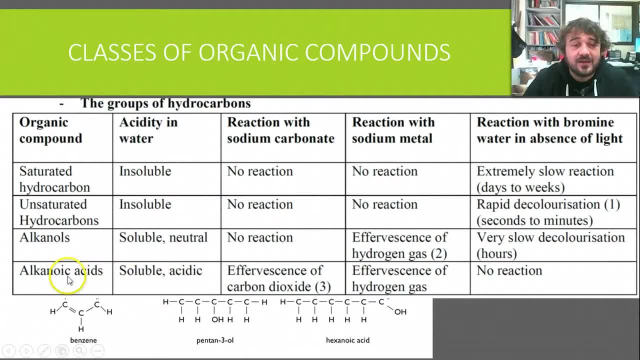 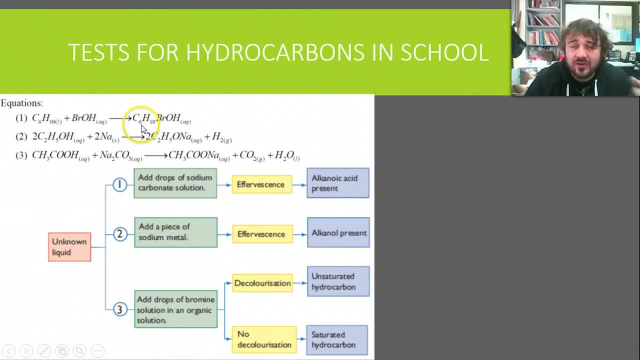 to work out exactly what it is. they're soluble and they're acidic duh, all right. so how do we test it? so here are your equations. these are good, good like. you need to know examples of these equations, and this is a nice little flow chart, again from your textbook on how to do it. so we 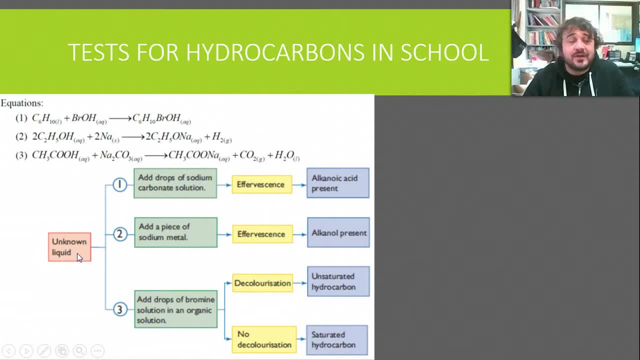 have another liquid. what do we have? what is our sample? this is one we can do in schools. you wouldn't necessarily. you would probably do this if you had a very large sample um in a lab to save some time. um, so we have our. i've lost my mouse there. it is all right. so we've got unknown liquid here. 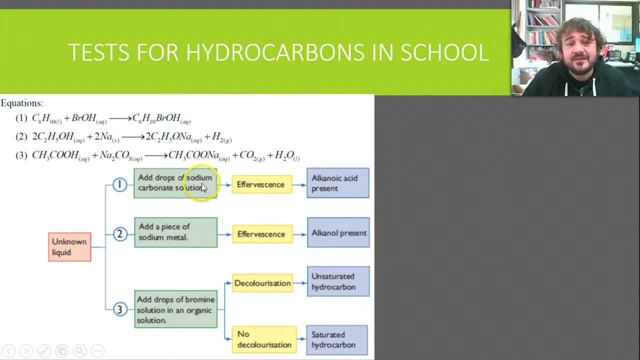 we could add some sodium carbonate. if it effervesces, it is an alkaline acid. cool if we add some sodium metal. to be honest, this one is either a. it's either going to be a alkaline acid or an alkanol. but we added some sodium carbonate and it didn't react to that. so we now know that. 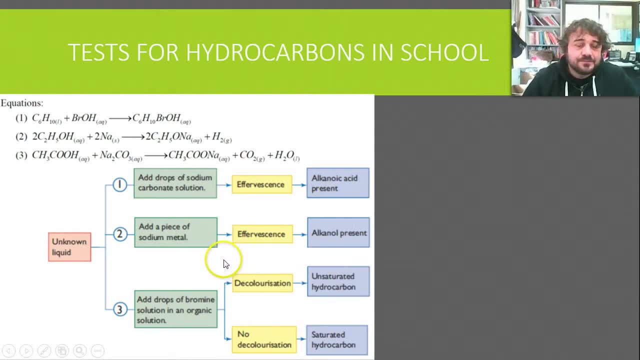 it is not this. it's an alkanol um doesn't react with either of these. we still don't know what it is. so if we add some bromine to it, um, if it decolor, decolorizes, okay, um, it is an unsaturated solution. if it does not decolorize. 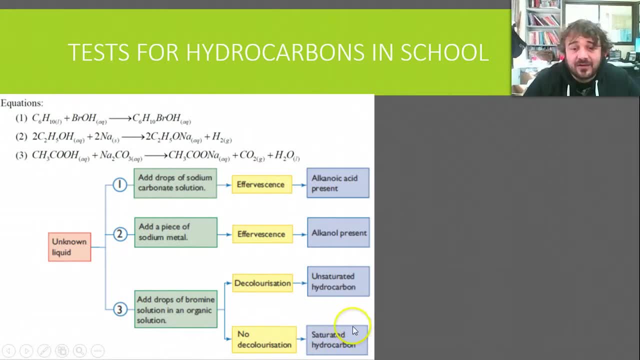 so if it stays the same in darkness, it's going to be sodium hydro, so it's saturated, so hydrocarbon. now, interestingly, this is obviously going to be a sodium hydrocarbon, so it's going to be a sodium hydrocarbon solenoid, so a fluoride test. so this is now going to have a lot of challenges. 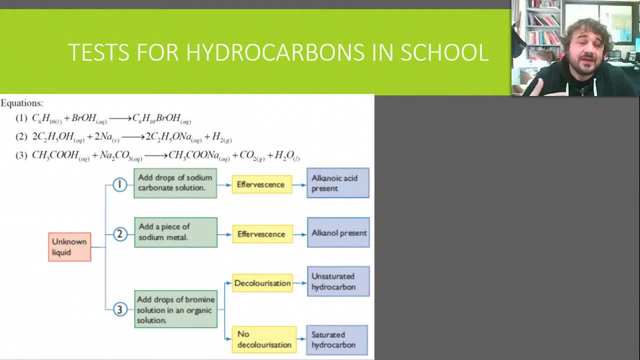 probably um important side effects, but it's a pretty common issue and this is a real problem. it's only been carried out for up to a balance of amounts and it's the only one that's going to do it, and it is not. it's obviously not the only tests there are. it is obviously not the only. 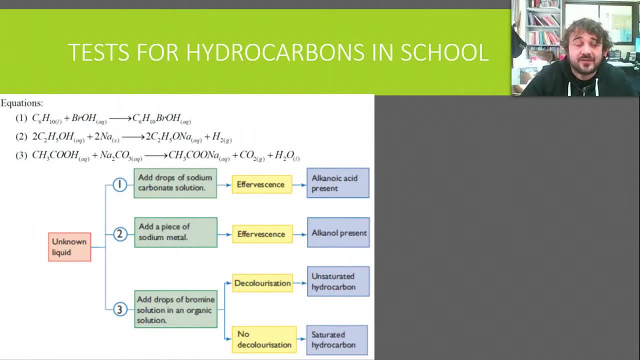 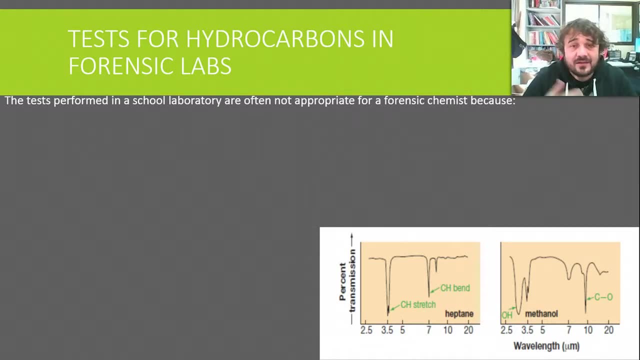 way to do it. however, they are the ways, which is, which are available to us in the school, and we'll do this in class. so that is not a complete list. clearly, that is just the list that we have. um, it's it's rare that you know you're going to find a very large sample. 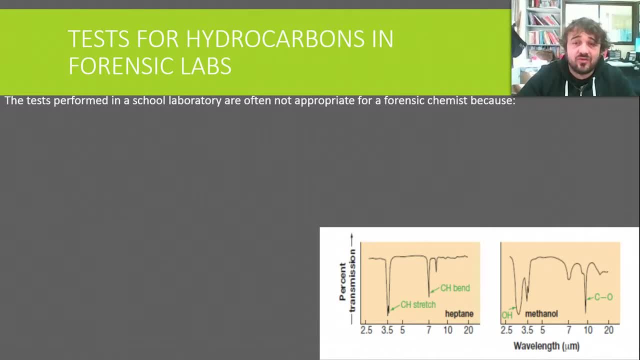 So the tests that we do in school: they're not appropriate for a forensic chemist generally, because our samples are often trace samples, so really small amounts, And they're not sensitive enough for what we need them to do. So sure, those tests will tell us it's a hydrocarbon. 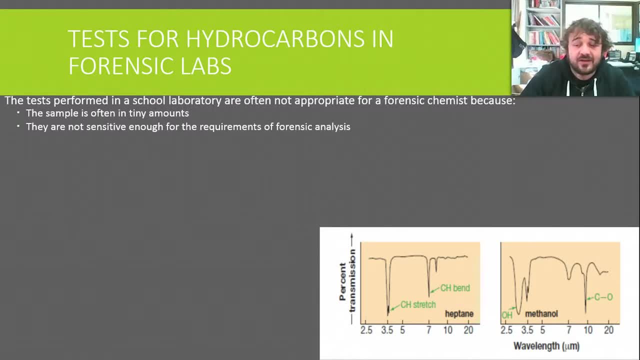 but it won't tell us which hydrocarbon or which unsaturated hydrocarbon. There are other ways we could do that in a school lab, but a forensic scientist. they get it a bit easier, So they do infrared spectroscopy. So it's very similar to AAS. 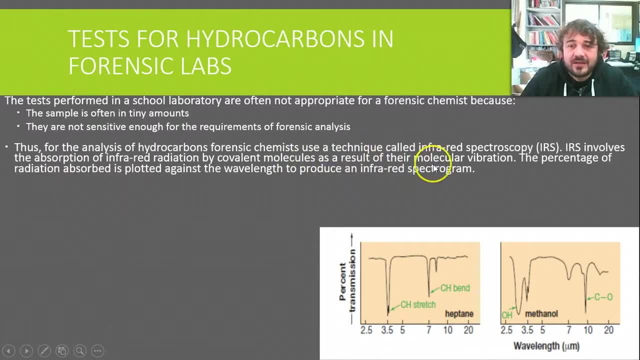 So we shoot infrared light through it and it's absorbed. It's absorbed by the bonds. So, percentage of radiation Now, each bond for the functional groups, the functional groups, each bond, each bond, each bond in the functional groups absorbs different amounts of light. 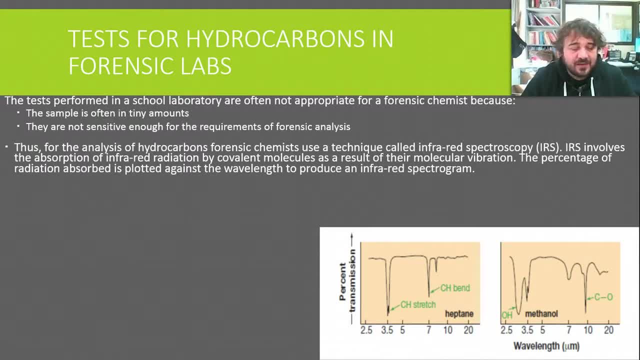 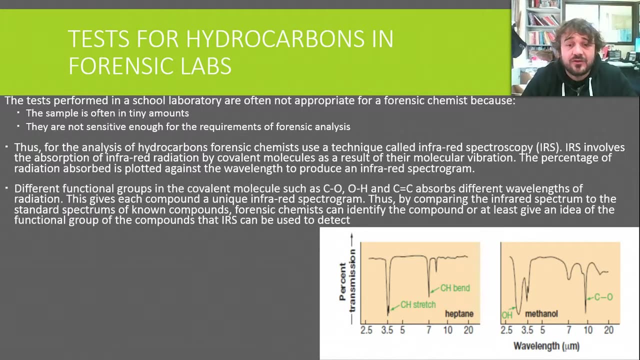 Okay, And because we can tell how much is being absorbed. we can actually usually tell how much is there, So it's a quantitative measure as well. So your different functional groups: they absorb different wavelengths of the radiation And this means they're unique. 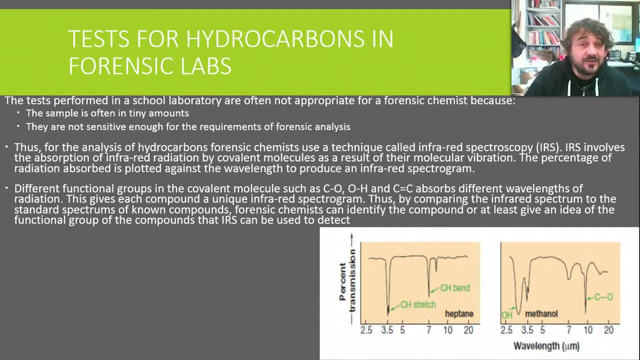 So, while even this is not a perfect one- remember we need to talk about limitations- here we can identify the functional groups of those compounds. There are other stuff we'll do beyond this, but we can now tell which of each of those functional groups is. 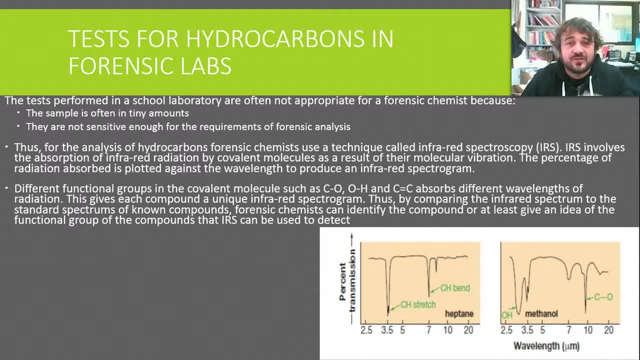 whether it's an alkanolic acid, whether it's an alkanol or saturated, unsaturated hydrocarbons. So it's really useful identifying carbohydrates in these ones. And you'll see, here each one has a. they'll have their own individual signature. 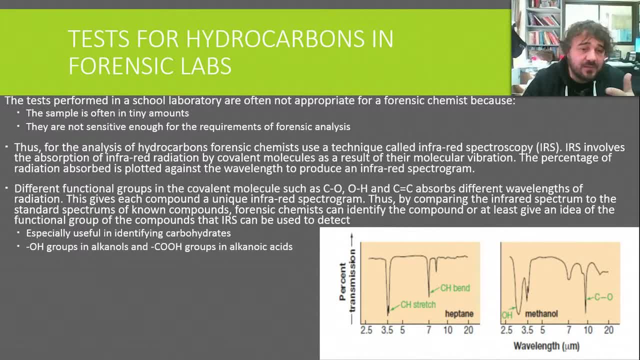 We can also use it to identify the. so we can use it to identify actual carbohydrates. That's actually not so hard to do, But the OH groups and the alkanolic acids, they're a bit tougher to identify what chain it is. 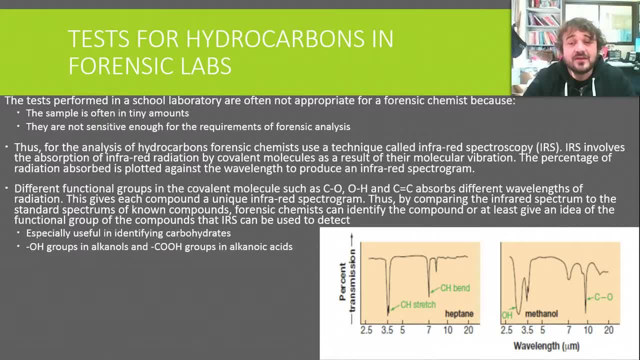 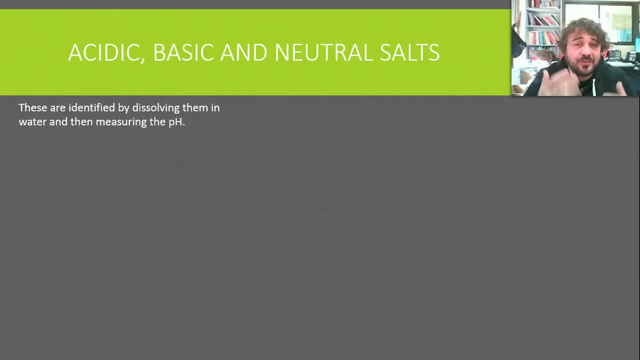 or what, the length of the chain, but we can still identify that it has certain groups. So, yeah, All right. So acids, acids bases and neutral salts is pretty much the same in both situations. So you dissolve the salt in the water and you measure the pH. 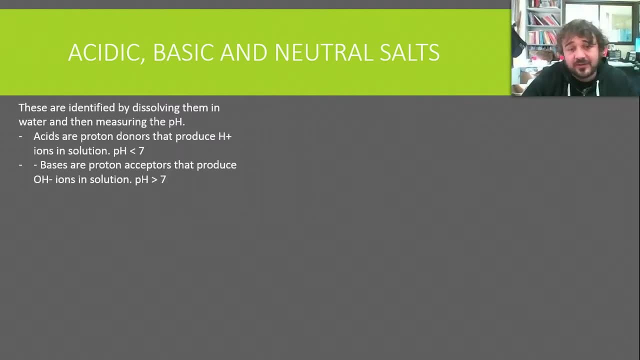 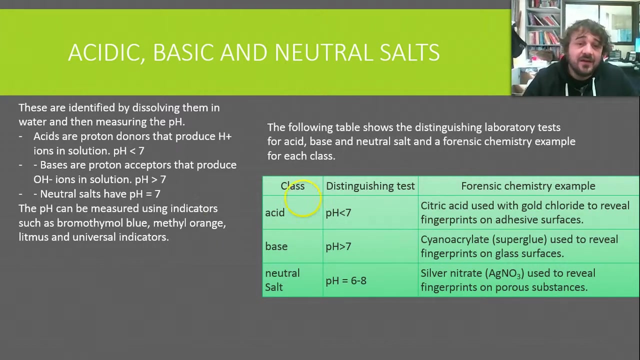 Acids, proton donors- pH less than seven, bases, proton acceptors- pH over seven and neutral salts over pH of seven. So we can measure these using indicators like bromethyl, blue, methyl orange, litmus universal indicator or a pH meter, for that matter. 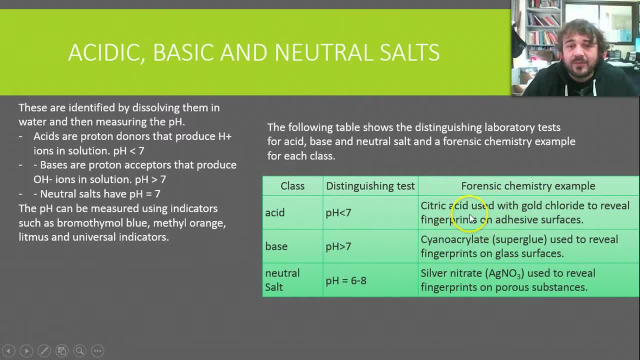 And over here we actually see where we we use different acids and bases in in forensic. This is just for interest. It's actually, I know, know that it's more than just for interest. It's useful, but that's why that's there right now. 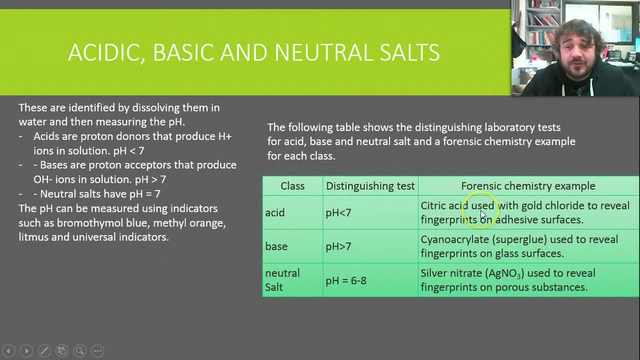 It's not the most important thing. So we use citric acid to reveal fingerprints on adhesive surfaces, Cyanacrylate- We use that to reveal fingerprints on glass, So they basically they vaporize the superglue over it- and a neutral salt, silver nitrate. 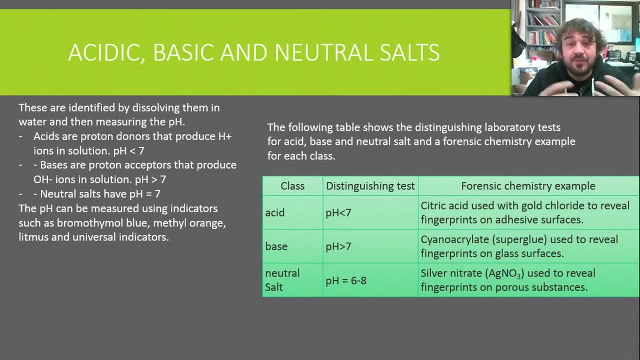 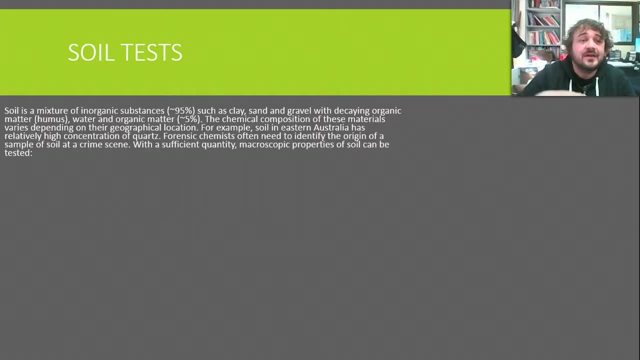 We use to um, try the fingerprints on porous substances. All right, now we're about to finish off with soil tests, So we've got two more slides hanging there. We're almost done. Um, so what is soil? It's basically. 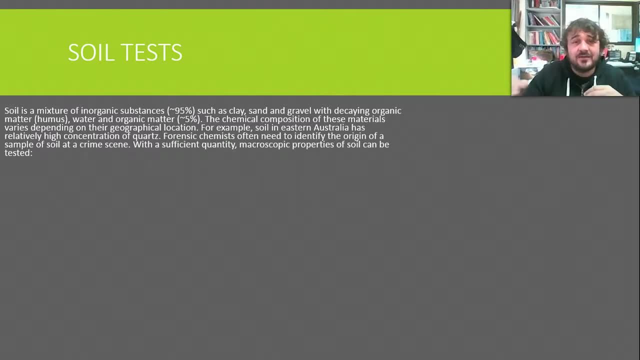 it's a loose mixture on top of the, on top of the, the ground, on top of the surface of the earth. Um, some geologists, particularly soil scientists, get really upset when you use the word dirt like it really upsets them. 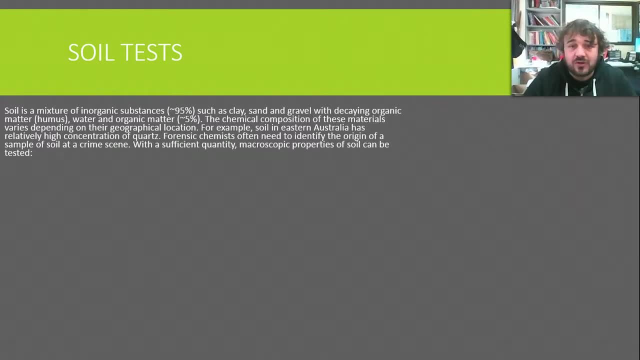 So if you know any of these people caught dirt, really it upsets them, Um, but essentially it's like 95% inorganic matter, Um and this. so we're doing clay sand, lots of silicates, that sort of stuff. 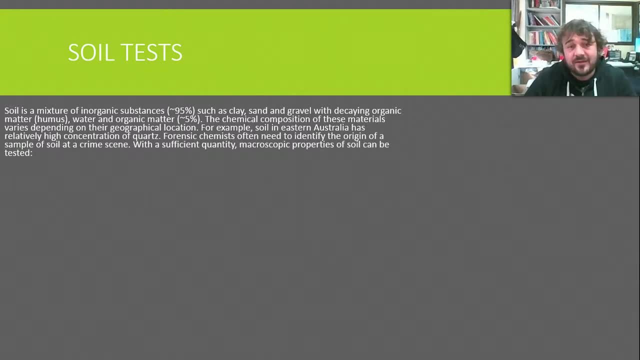 um gravel, and then it's got decaying organic matter or organic matter mixed into it. Um, I don't know why it says hummus. Um, so water, organic matter and so forth. uh, breaking down leaves. the chemical composition of these varies depending on the geographical location. 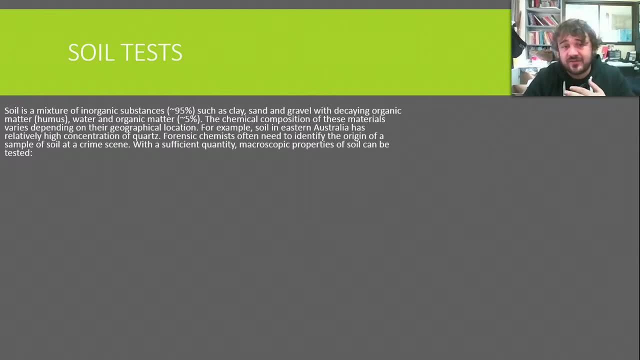 And all right. so if you're in the Eastern half of Australia, it's got high concentrations of quartz. but but what's even more, it's more specific than that. So the soil on one end of town is going to be different to the soil in a. 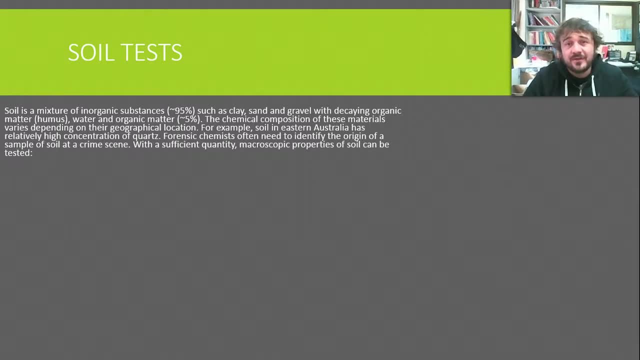 different part of town. The soil changes as you move within. you know several hundred meters, So soil is highly variable, but it's also highly distinctive for a certain area. Um, so there are several physical properties. we could test macroscopic properties. 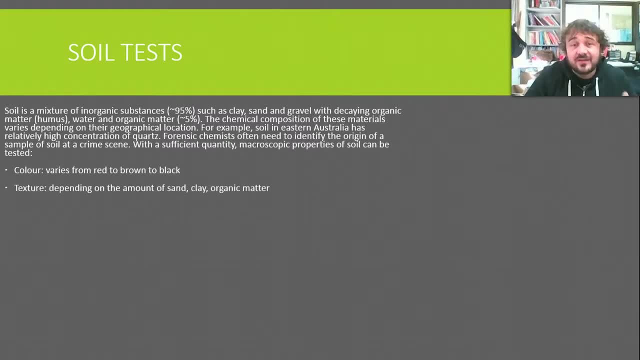 probably, as we can see. So color, um, texture, So it's like this is a thing. It sounds a bit wishy-washy, but if we've got enough of it, we can actually test the texture, texture, And there is a somewhat arbitrary but numerical way to do it. 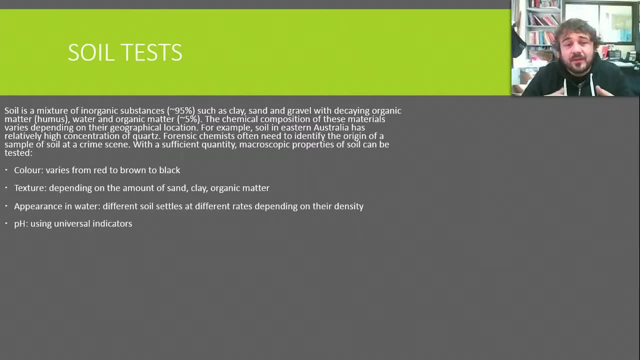 Um, we can see it. has it look in water? Um, the pH. you could use all of those to put together a profile and then compare it with a profile from another area and see what you've got Like. see if it's the same deal. 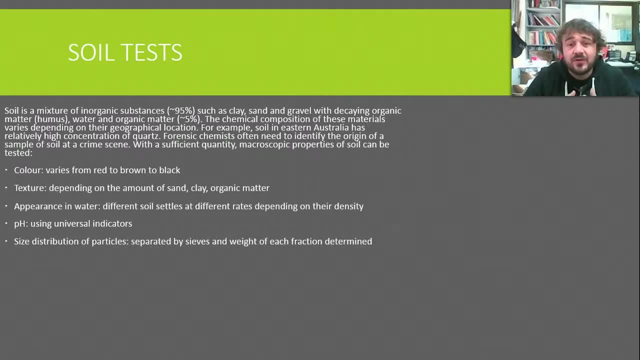 Um you also the size of the particles? Um, if you get a hundred grams of it and you run it through different size sieves, you work out which fraction is each. that should be fairly consistent for soil in that close area, especially at certain heights. 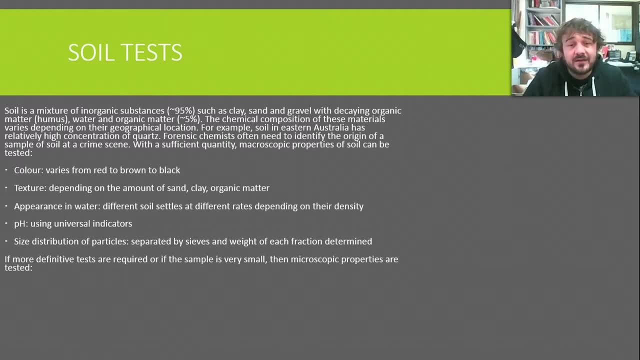 Um we, if we need more definitive tests, or if we've got a? um, a very small sample, then we can test the microscopic properties. uh, pollen, what pollen is left in the area, the specific for the plants? 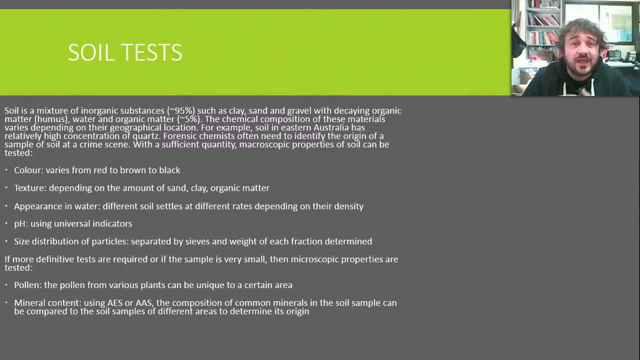 um the mineral content. So we do AAS and we can work out the composition of minerals in the soil as well as the amount of those minerals in the soil. So that's pretty sweet. Um glass fragments. glass varies widely. Um. 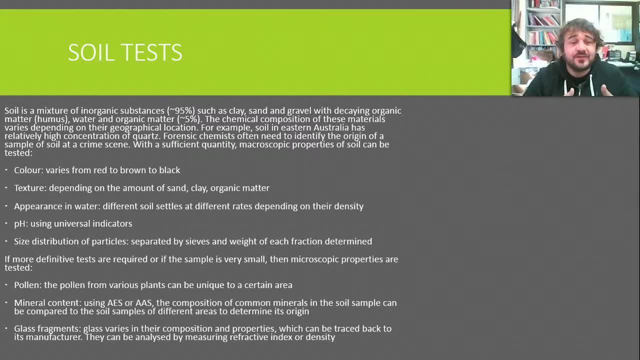 but the composition of properties is usually very specific to its manufacturer And, to be honest, very specific to the particular factor. So if you've got a particular factory, so if you've got one manufacturer but there's a separate factory, the glass properties will be different at different factories. for the 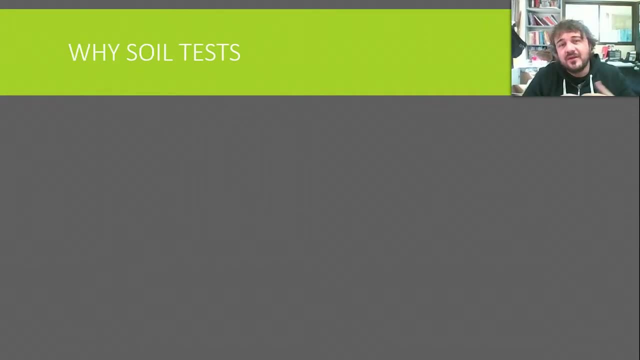 even though they're going to use roughly the same composition. So why do we do soil tests? Basically, that many, many applications, uh, footprints. we can show that the perpetrator came from a particular location. However, um, you can match the soil from a footprint with the bottom of the soil. 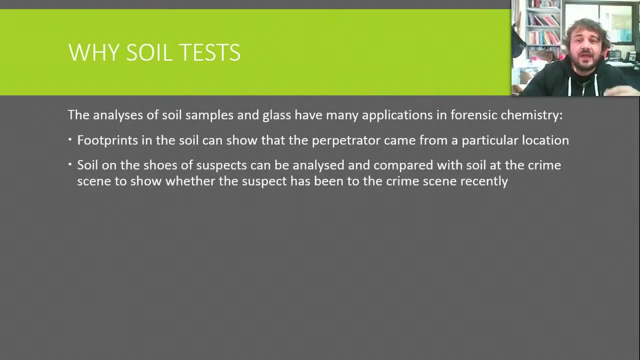 the bottom of a shoe, Um, and it says here- and that could confirm it, This doesn't just be shoes, This means other bits of equipment that will have dirt on it, Soil, sorry, Um, last fragments which is found in soil. 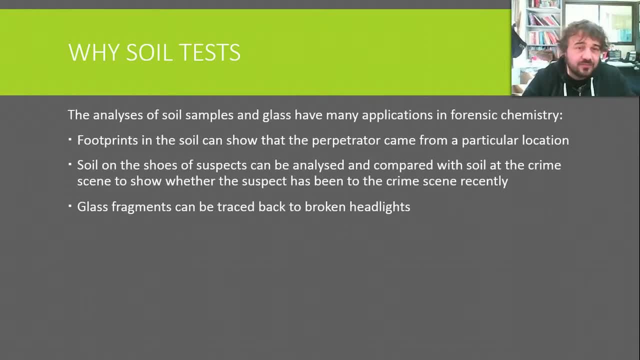 Um, again, we can track it back to broken headlights, to also any glass where you want, Really, Um. one thing that's starting to come up is the glassware from phones. in a violent crime, phones break And because of the mass production of these things, 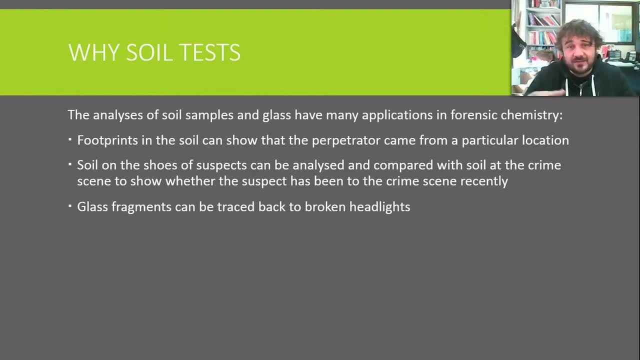 the glass from the gorilla glass that it's on the cover of most phones. it's fairly specific to kind of the day and the time it was manufactured in the factory, So you can actually usually pinpoint with some degree of certainty if it's come. 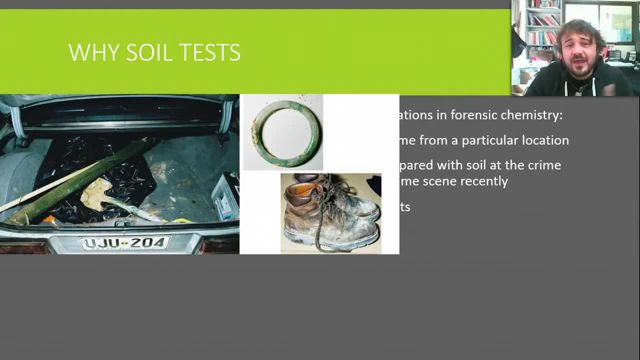 from a certain phone. Anyway, that's interesting. Um, so here we have some evidence from a real murder case. Um, this is from South Australia. There was a- uh, we don't get the details of it. Um, a guy was pulled up. 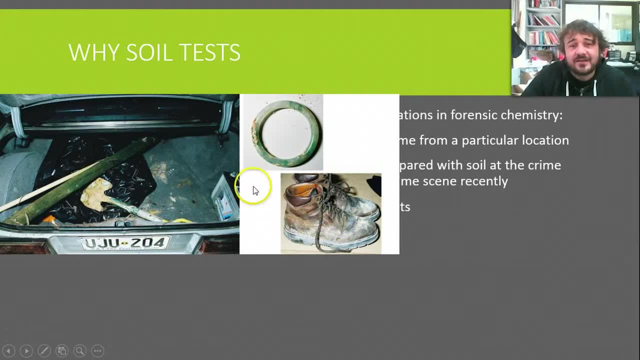 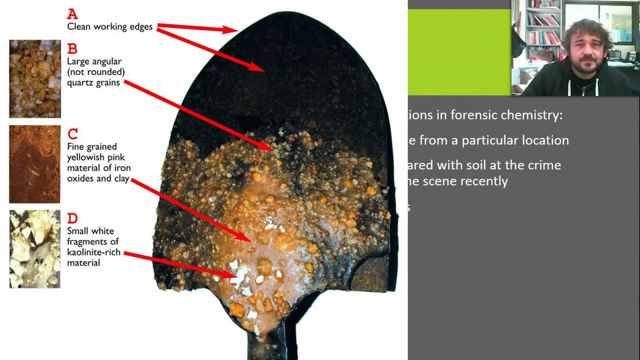 pulled over and he had this stuff at the back of his car, as well as the car. That's a certain description as well as these are issues. Um, if we look at his shovel, we can see what's been left on his shovel. 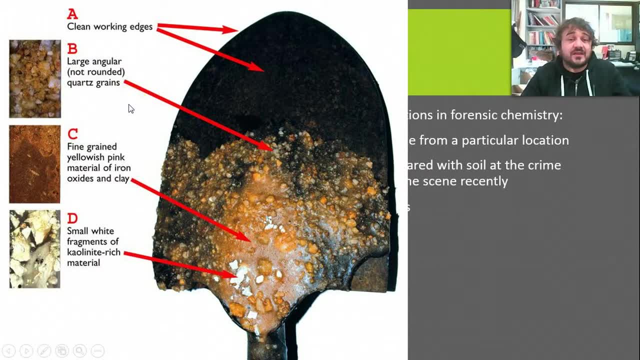 Okay, This stuff here can be used to work out the composition of the soil where he was digging And we can compare this to where the body their family was buried. Um, so yeah, like it's really useful, the soil stuff. 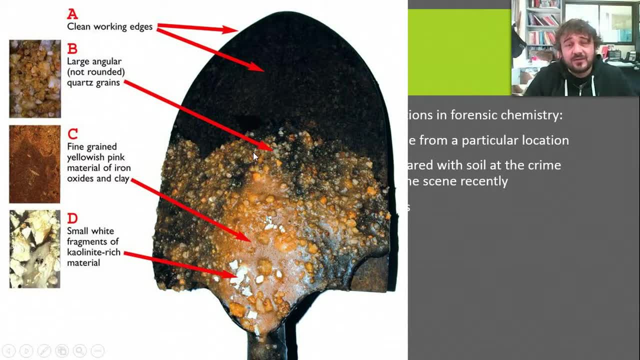 And remember we could do it if we want on a very. you know, if we've got a large sample, like you'd have here when you do the really simple stuff, which is still very reliable, Um, if we only have a small sample, 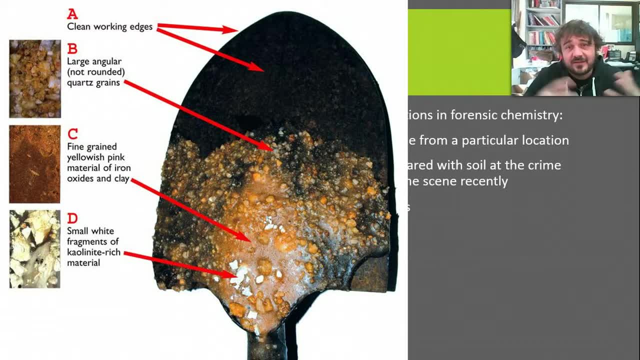 then we can do the smaller stuff, which takes more time. So the AAS and so forth. Um, so you can use the shot. We can link this shovel to where it was used to dig a hole in ground. Does this? does this mean that the person who owns the shovel, as the shovel buried, the 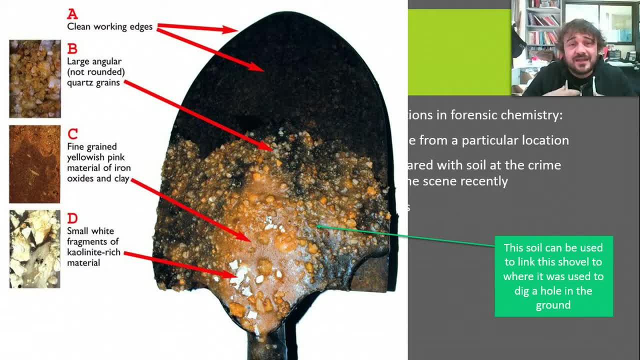 body that's in that ground. No, all it actually means is they dug a hole somewhere nearby where that certain body was found. So now I've got one piece of evidence and I want you to really get your get a grasp on this is if there's one piece of evidence. 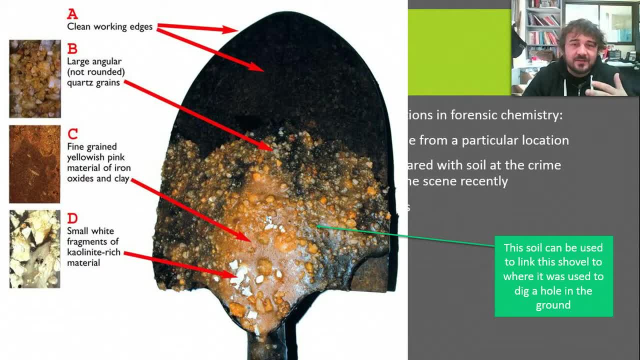 this is not a smoking gun. This means this helps build up a larger picture. The idea of forensics is not to go. here's your picture. Here's a piece of evidence that convicts done. The job of forensics is to build up a picture. 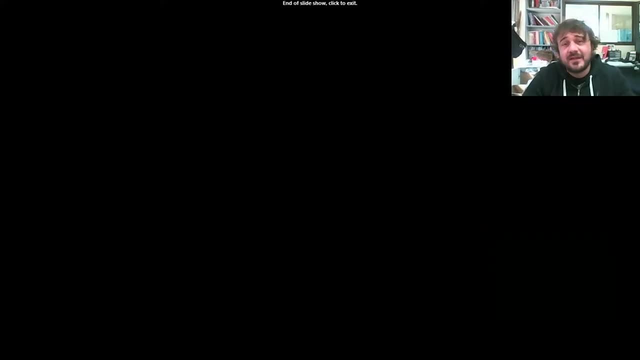 build a larger picture of what happened in a scene of crime. Um, and that's it, And I'll see you in class.